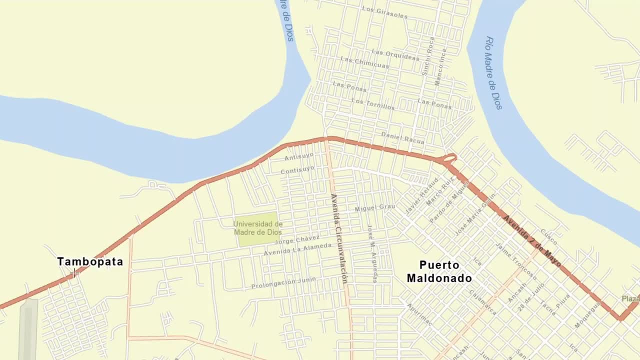 At number one, we're going to look at the role of data management in GIS. Data management in GIS is the process of organizing, storing, retrieving and maintaining geographic and attribute data. GIS data consists of either vector data or raster grids. First, 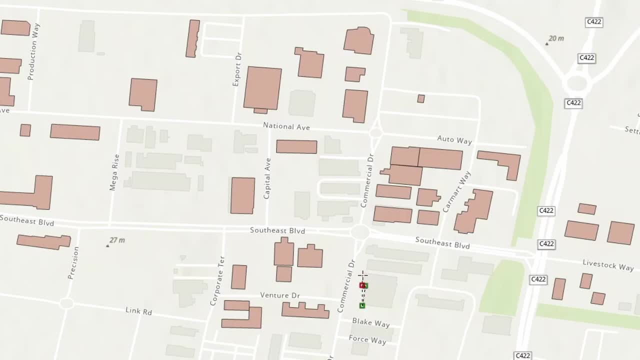 vectors are points, lines and polygons with vertices. For instance, administrative boundaries are often represented as polygons, whereas something simple like fire hydrants is stored as points. Roads are administrative boundaries and roads are administrative boundaries. Roads are a good example of line data. The other type of data type is raster, For example, satellite images. 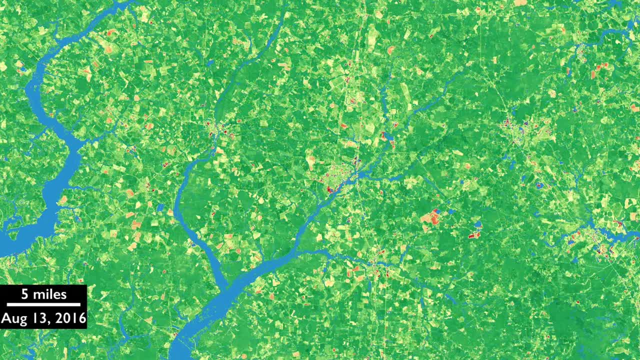 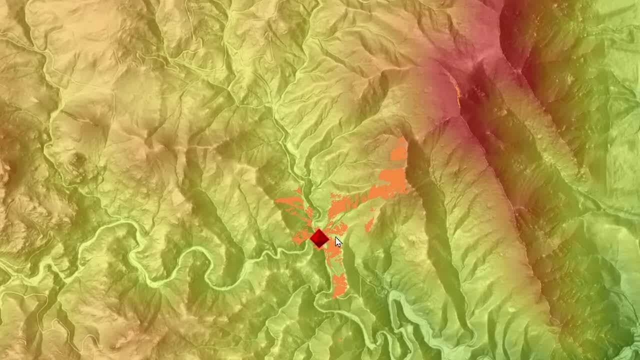 aerial photographs and digital elevation models are examples of raster data. We also call it grid data because it's represented as rows and columns. We use these two data models every day in GIS. Each type has its own strengths and weaknesses and is better suited to different 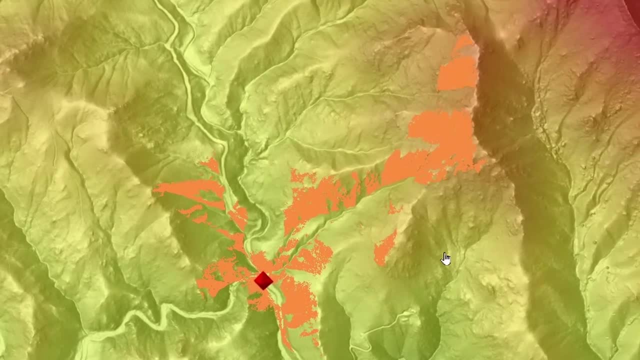 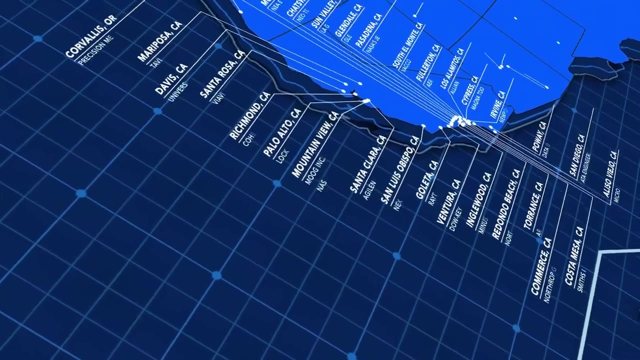 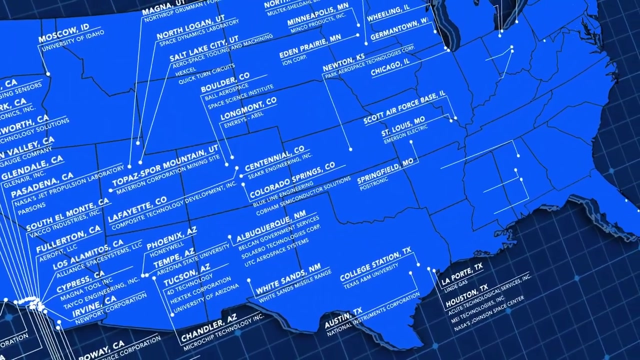 kinds of spatial data and analysis. At number two we have visualization. Let's say you have a latitude and longitude coordinates in a table. I think you can agree that it's really difficult to know where those locations are. But once you show the data on a map it provides geographic 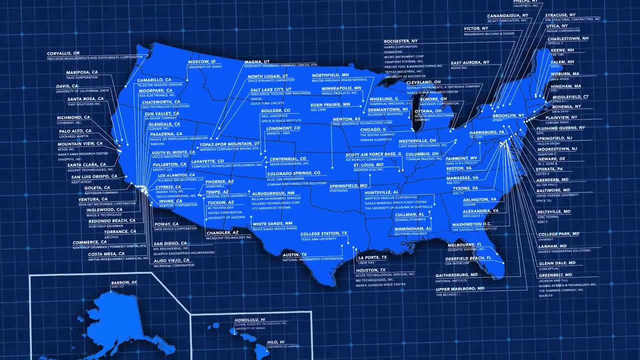 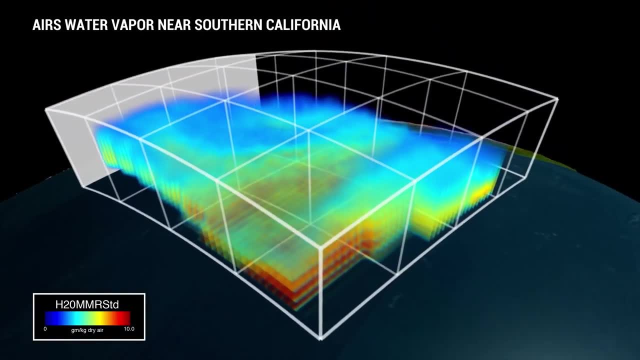 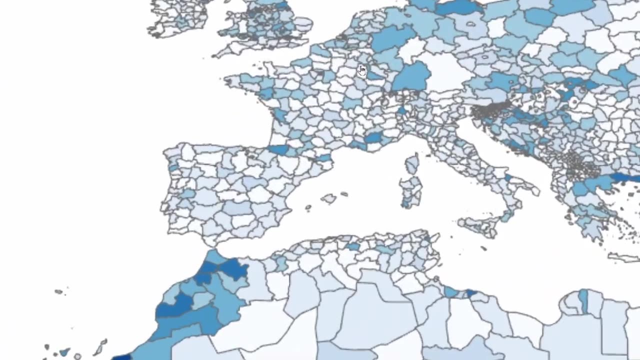 context, so you can fully understand where these locations are in the real world. GIS works with these physical locations instead of tables, And we map it all out. Here are some of the most common types of maps: Coropleth maps use shading or color to represent data values for different regions or 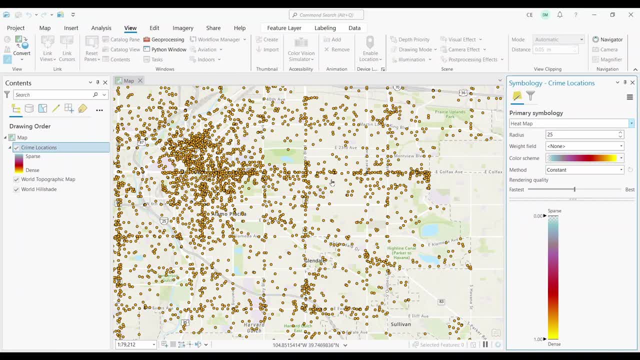 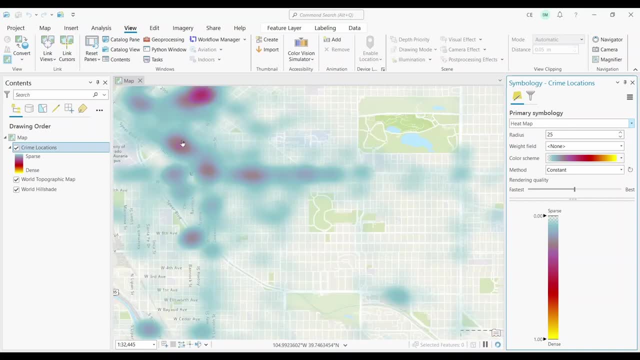 visualizing demographic or socioeconomic data. Heat maps use shading to represent the intensity or density of data values in an area. Heat maps are often used for visualizing spatial patterns in data such as crime or traffic density. An isolene map is a type of map that uses contour. 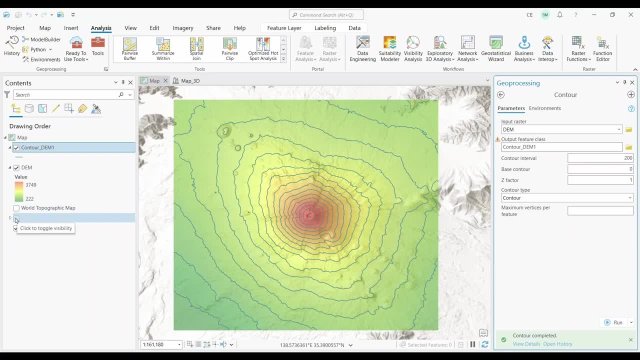 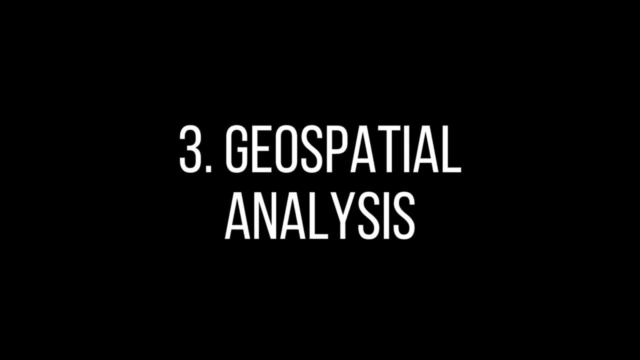 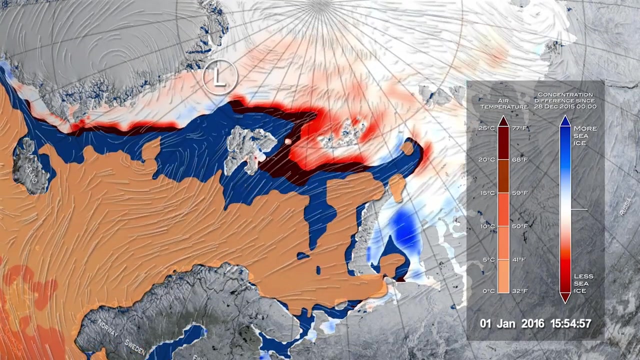 lines to represent data. They connect points on a map that have the same value, such as temperature, elevation or rainfall. At number three, we're going to look at geospatial analysis. The purpose of GIS is to analyze geographic relationships and patterns using geoprocessing. 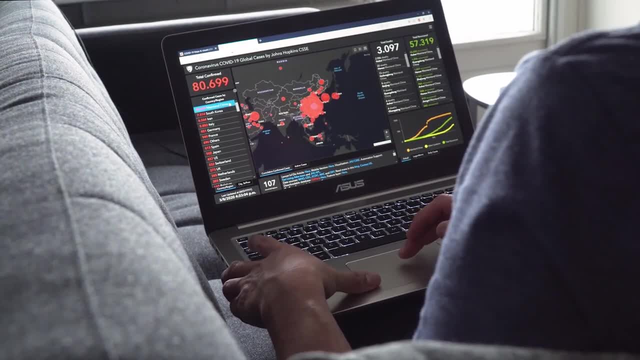 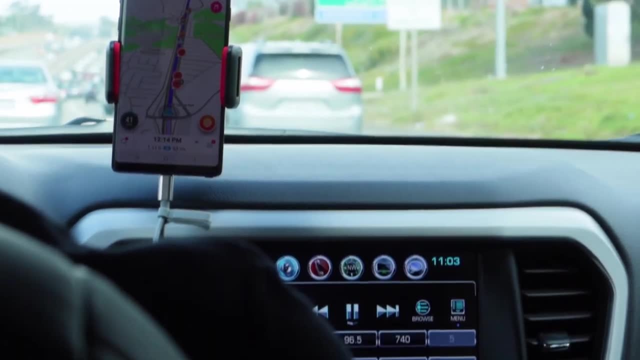 Geoprocessing can be used to perform a variety of tasks with a focus on extracting meaningful information from geographic data. For example, a GIS can identify the shortest route between two points, or it could create buffers around features. It can also overlay different data layers to 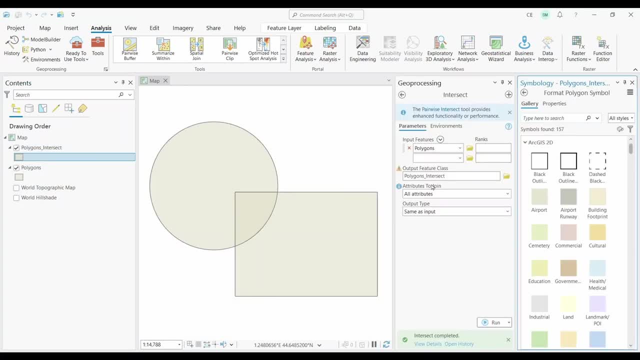 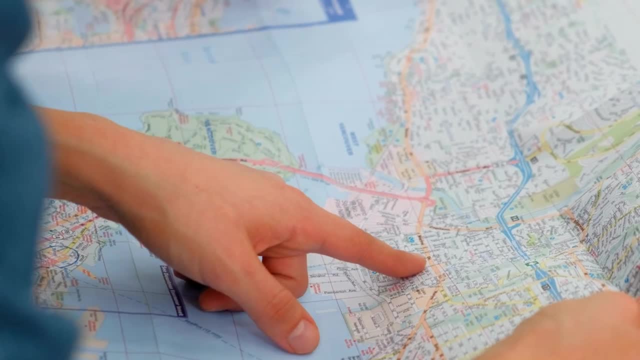 identify spatial relationships and conduct statistical analysis on geographic data. They say you don't truly know your data until you're in the field of geospatial analysis So you can visualize and analyze it geographically. Through spatial analysis you can solve location. 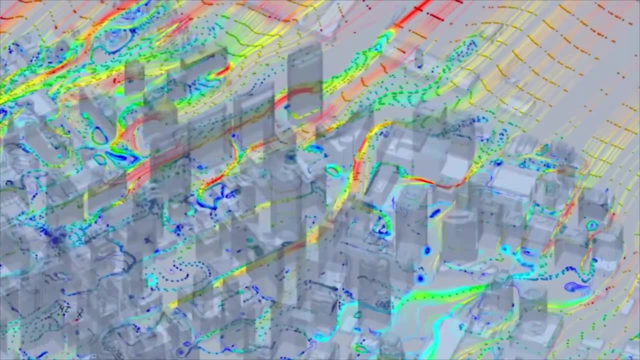 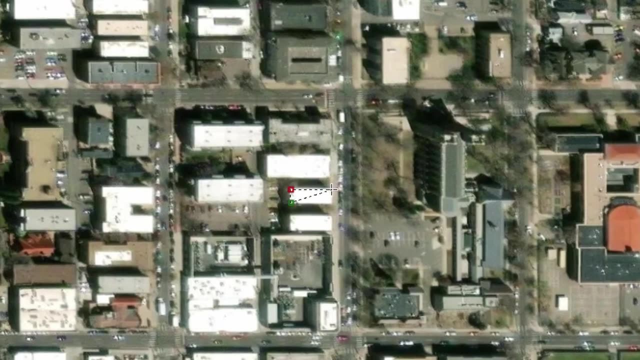 problems, to measure, quantify and understand our world better. And finally, at number four, we're going to look at the role of GIS editing. GIS data is a key component in the development of accurate and effective applications, Because without geospatial 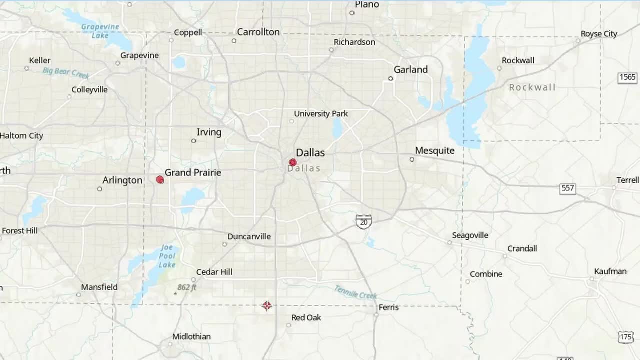 data, the field of GIS wouldn't exist. Editing involves building new data sets from the ground up, including existing geographic data. It's important because it ensures that the data being used is accurate, up-to-date and relevant to the problem at hand. 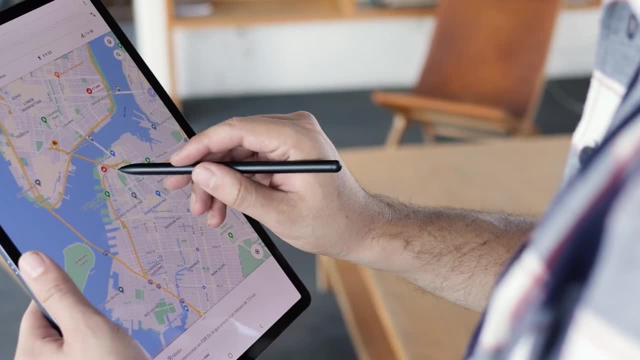 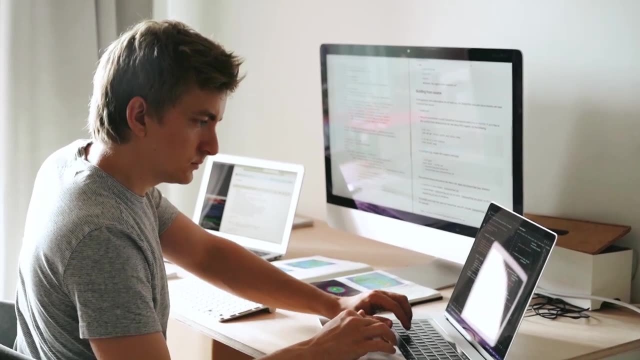 Now that you have a bit of background on what GIS is all about, let's take a closer look at some of the most common types of GIS jobs. If you're just starting out in the field of GIS, you'll likely start as a GIS technician. This role involves most of the grunt work, like data editing and map. 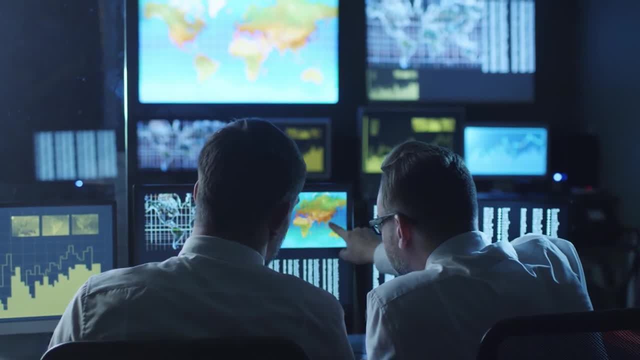 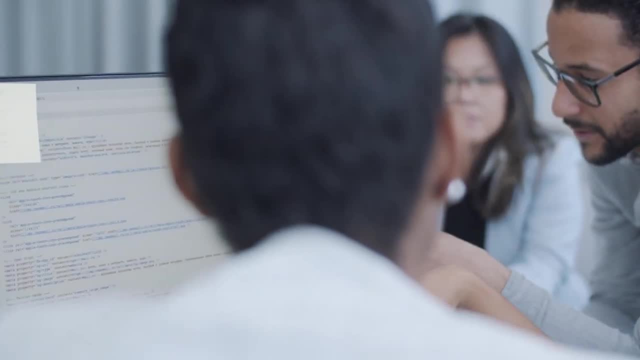 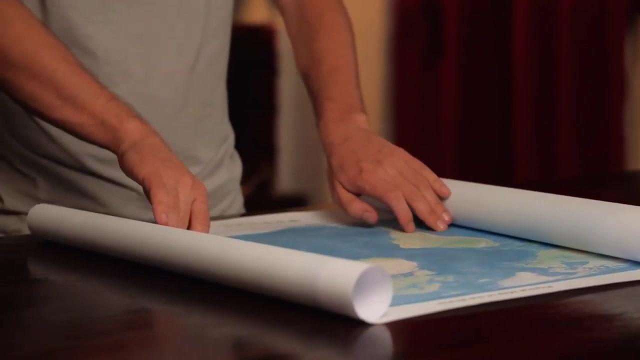 production. You'll often find that the most common role is either a GIS analyst or specialist. Both types of roles typically are heavily involved in geospatial analysis and it may involve data modeling and coding. Another common job in the GIS field is a cartographer. Cartographers specialize in creating 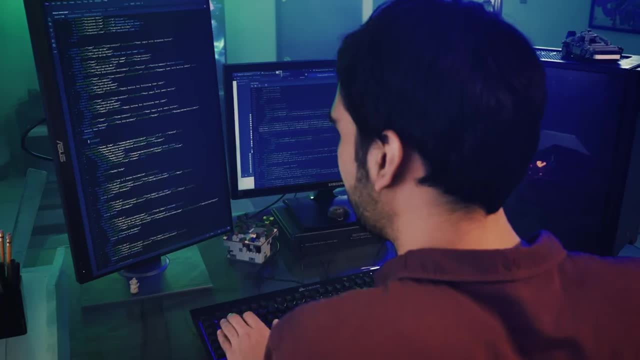 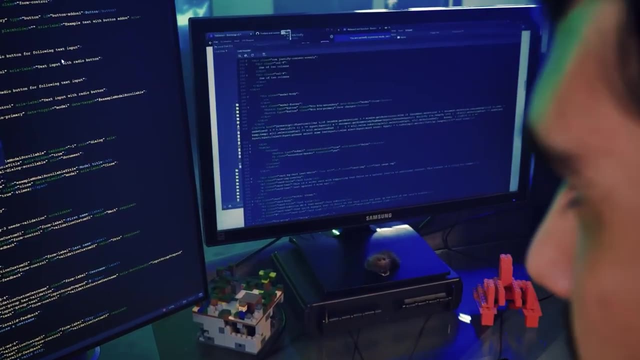 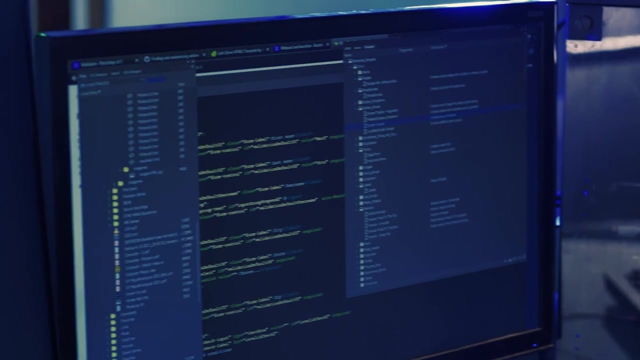 visually appealing map products and communicating this information. Finally, GIS developers strictly work at code development. This might be for the purpose of automating workflows, of building customized scripts that perform a specific task. seen its fair share of twists and turns, GIS has steadily increased in demand and is becoming more. 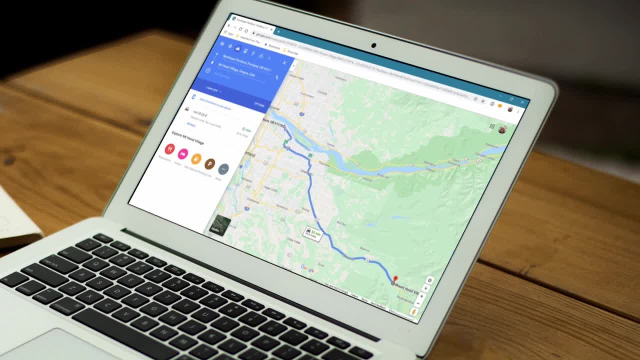 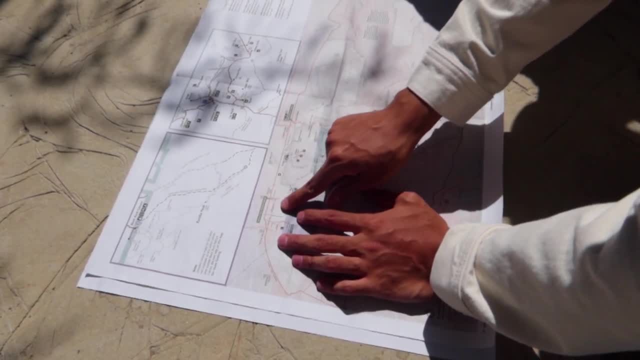 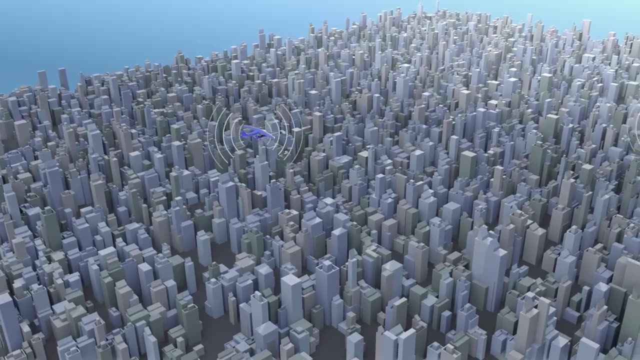 mainstream in various industries around the world. We use GIS in a wide variety of applications across many different industries. Here are some of the biggest users of GIS: Urban planners use GIS to model and analyze urban land use, transportation and infrastructure. This helps planners make 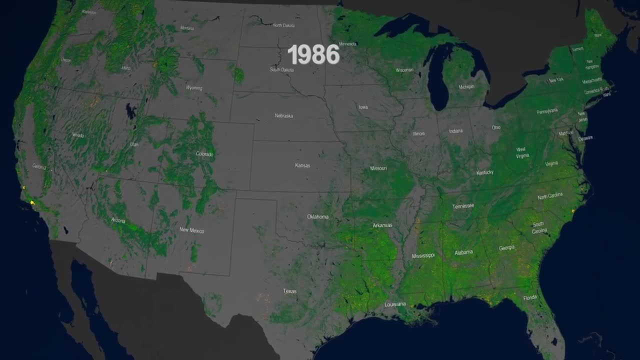 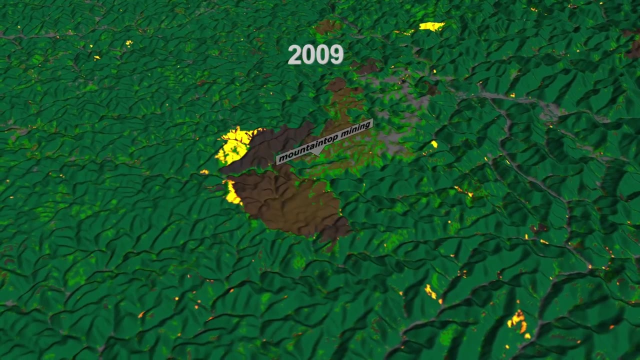 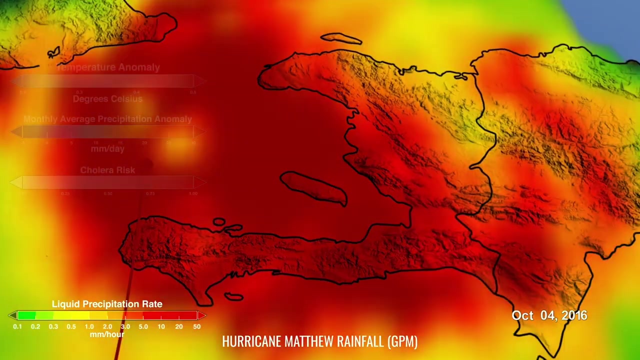 informed decisions about development and growth. Environmental management leverages GIS to monitor and manage natural resources, track species, habitats and predict the effects of climate change. Emergency management uses GIS to manage and respond to natural disasters, disease outbreaks and other emergencies. Marketers use it to help businesses target their marketing efforts. 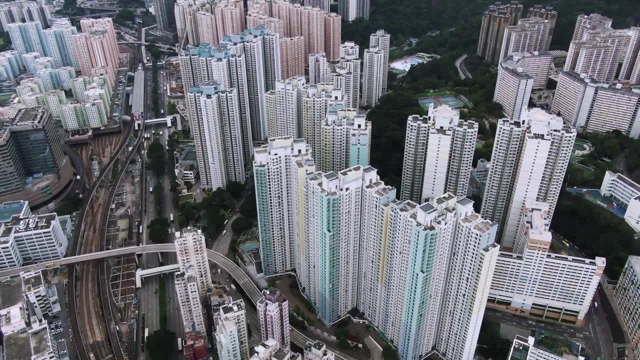 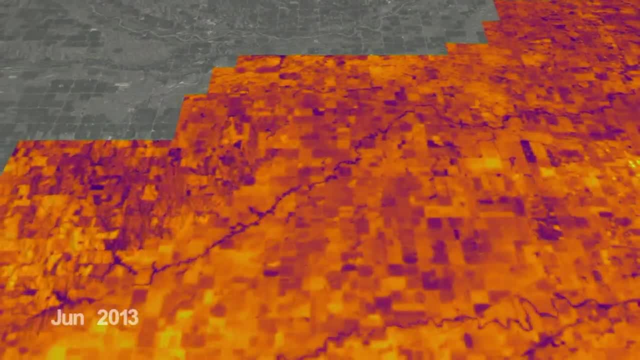 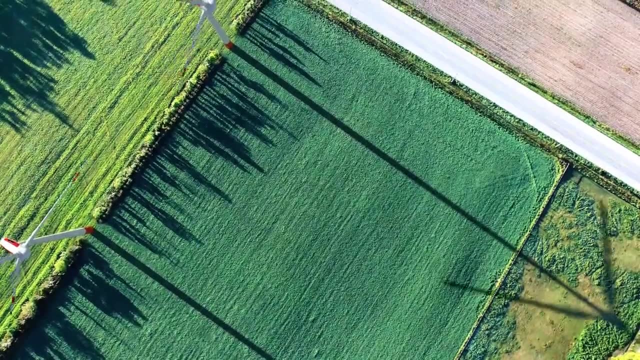 by analyzing demographic data and consumer behavior patterns In agriculture, GIS can optimize crop yields management, manage land use and monitor soil and water quality. In energy management, we use GIS to manage and optimize energy distribution networks, monitor energy usage and identify opportunities for 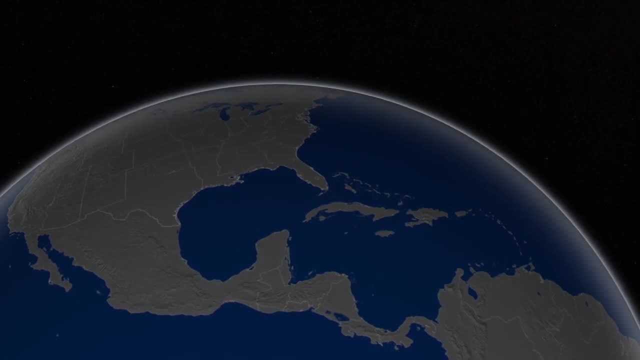 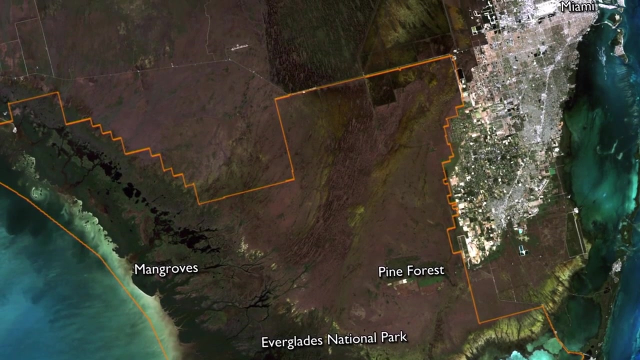 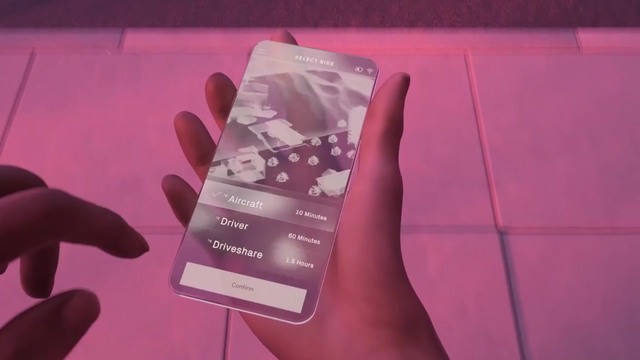 energy conservation. There are countless ways where we are using GIS to improve efficiency and make a difference in the world. As technology evolves, so does the entire industry of GIS. Here are some of its current and future trends. Mobile GIS has really been mainstream for a long time already Because of the increasing use of smartphones and tablets. 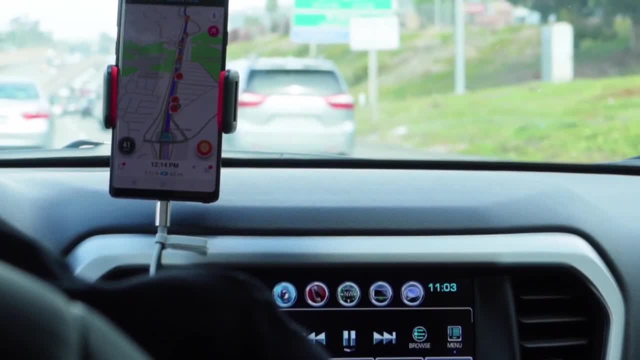 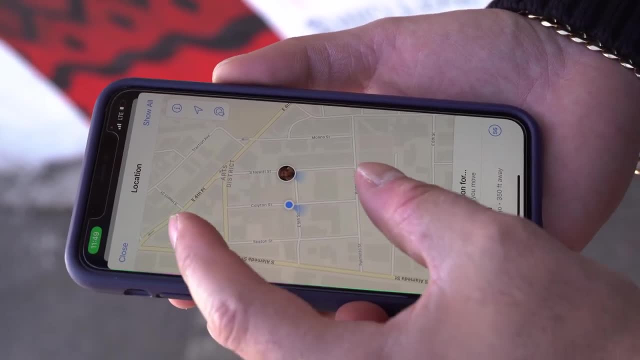 mobile GIS enables users to access and interact with geospatial data from anywhere using mobile devices. This is leading to new applications in areas such as field data collection, asset management and emergency response. Open data and open-source GIS software are also mainstream now. 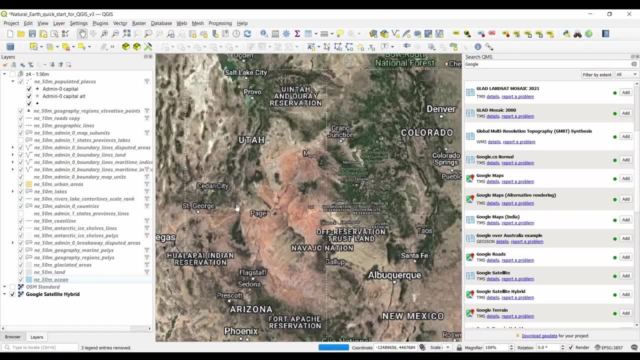 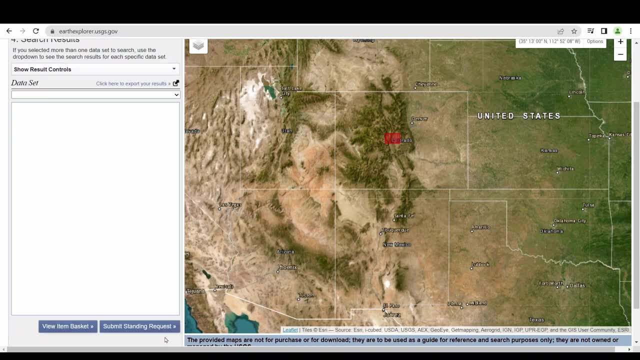 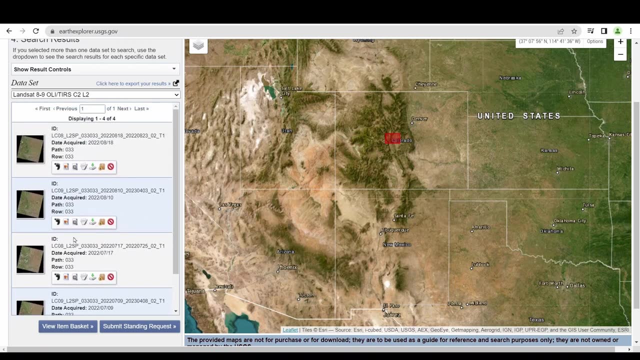 Open-source software like QGIS provides access to a wealth of geospatial data and tools at little or no cost. In addition to open-source software, we are seeing more open data portals, which are common in all levels of government. Cloud-based GIS services allow users to store, process and access geospatial 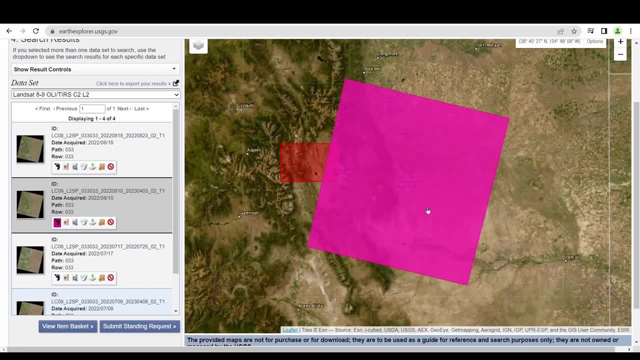 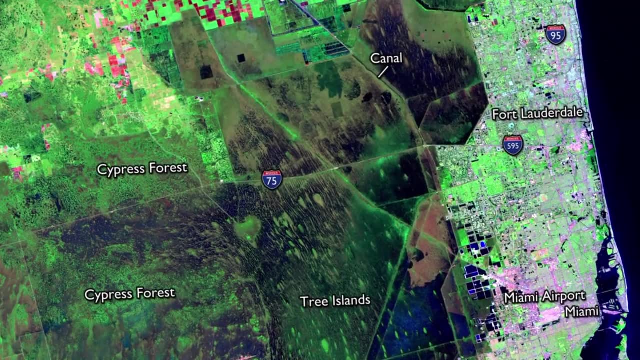 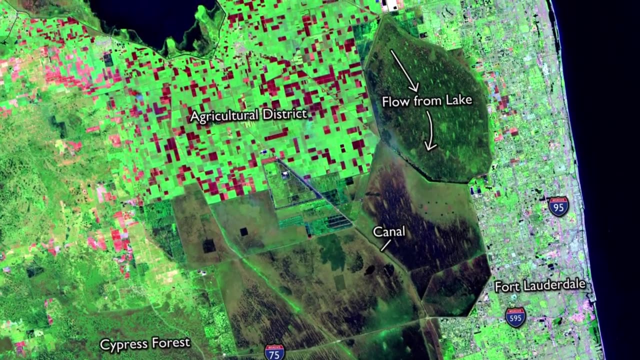 data in a highly scalable and cost-effective manner. Cloud-based platforms offer flexible computing resources and easy access to a wide range of geospatial data. With the explosion of big data in GIS and the increasing availability of AI and machine learning tools are transforming the way we analyze and process data. We are now able to use GIS to analyze and process data in a wide wide range of geospatial data. With the explosion of big data in GIS and the increasing availability of AI and machine learning tools are transforming the way we analyze and process data in a wide 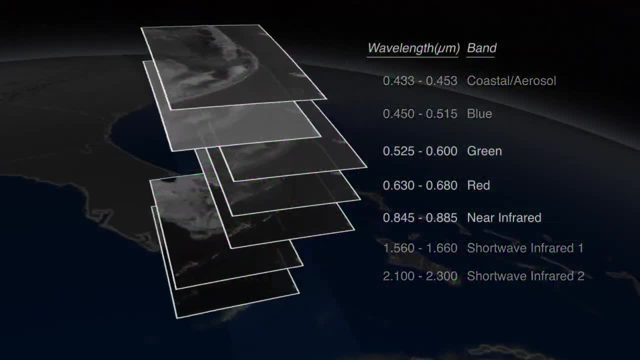 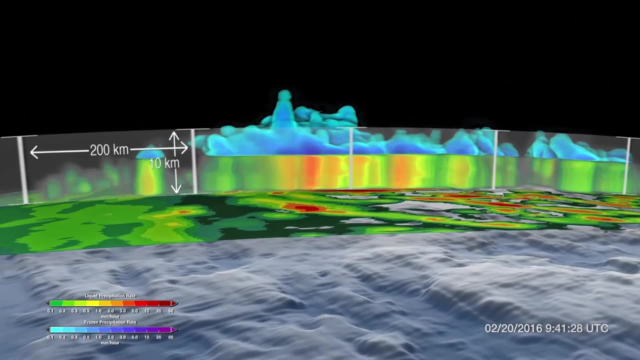 wide range of geospatial data. We are now able to use GIS to analyze and process data in a wide capabilities are helping to unlock insights from vast amounts of geospatial data. Finally, we have 3D data. With the increasing availability of 3D data and visualization tools, 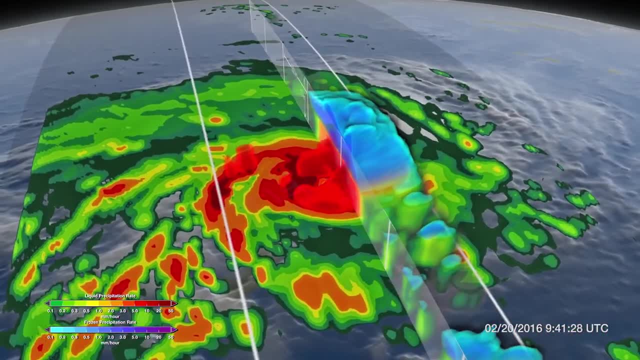 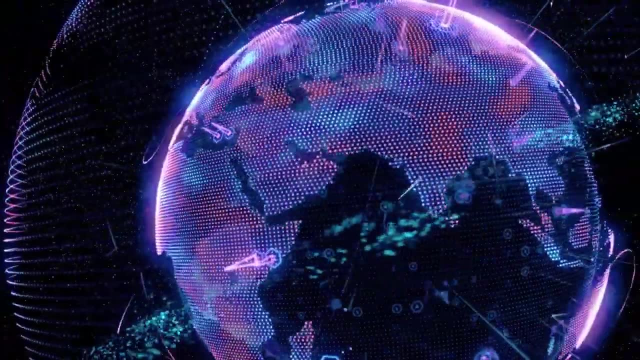 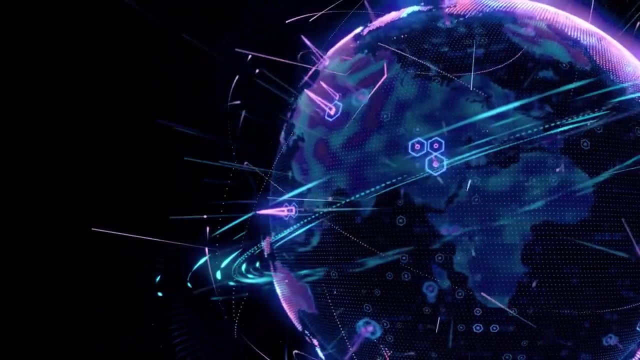 it enables users to visualize and analyze data in a more realistic and immersive perspective. Alright, There you have it. That was our definition of geographic information systems. Now we'd love to hear from you any questions you might have, you might have in the comment section below. Also, please don't forget to like and subscribe. to our channel for more great videos. See you next time.